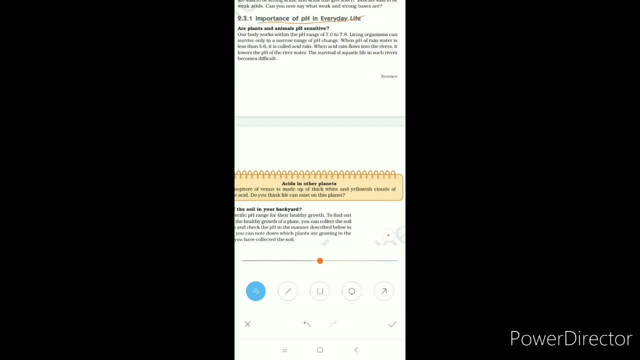 only in a narrow pH range of change if there is a high change in the pH level then the survival of the organism in the environment is facing problem or getting difficult so when pH of rainwater less than 5.6 then the rainwater is called the acid rain and this acid rain when fall on the rivers then it will lower the pH of river water there when it causes problem or cause problem to survival of the aquatic life as well as when it's fall on the soil then also it will increase the pH level of the rainwater and the survival of the aquatic life is reduced but when the pH of the soil as well as it will face problem on 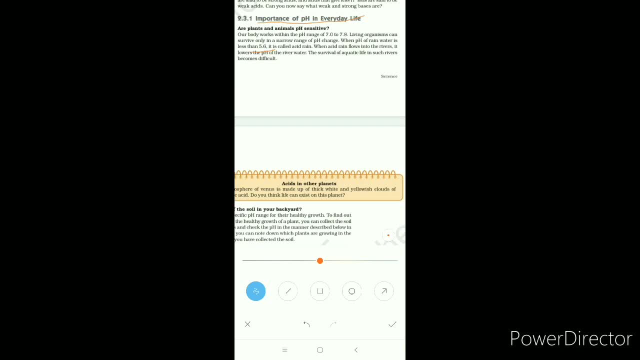 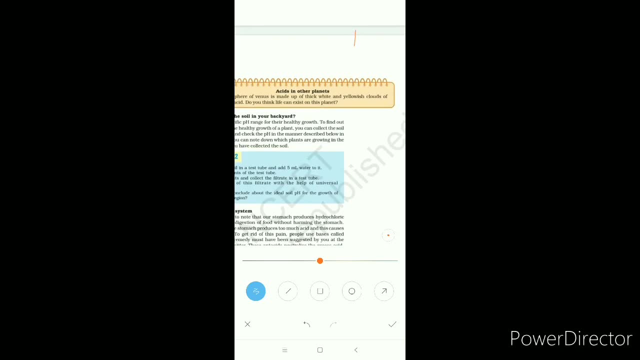 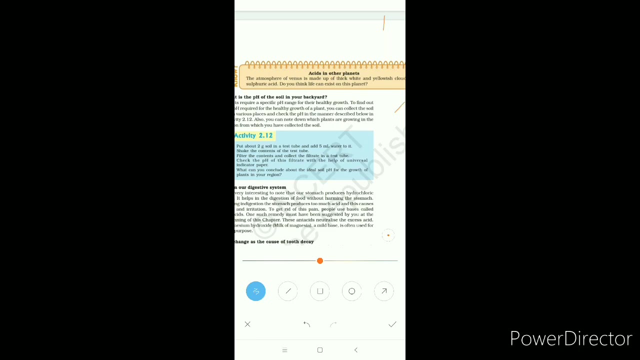 plants as well as some organism present in the soil so here retained acid in other planets so if we talk about the planets other planets then here the venous atmosphere is made up of different algae in different places as I mentioned we call them acid as well as it will face problem on plants as well as some organisms present 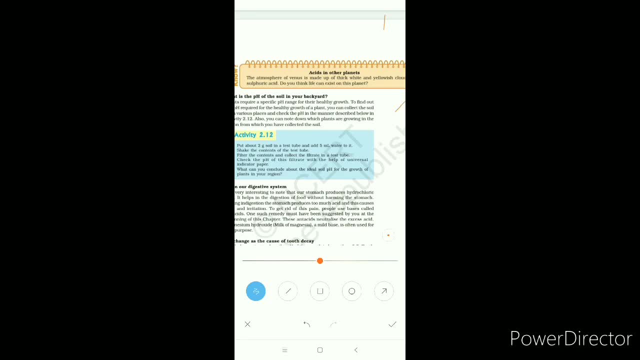 of white thick and yellowish color sulfuric acids so actually in venus there is most of the sulfuric acid and this sulfuric acids exist in the planet and because of this life existence is not possible in the planet venus 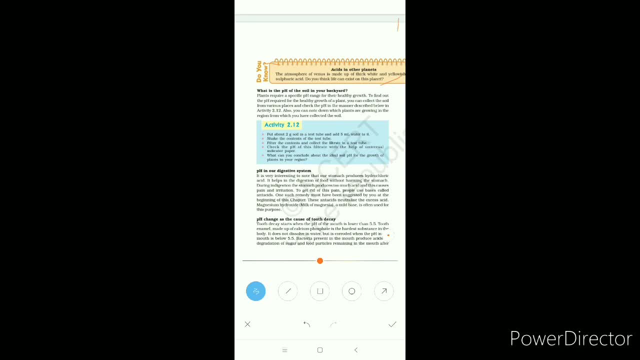 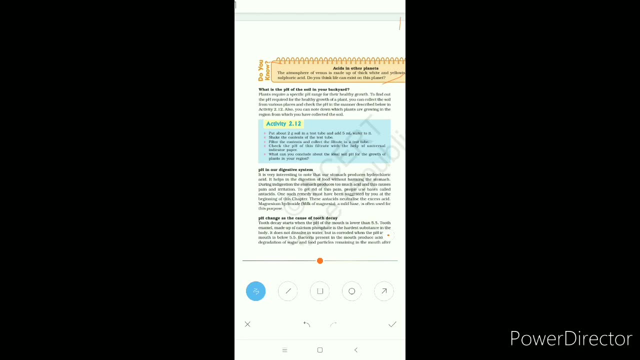 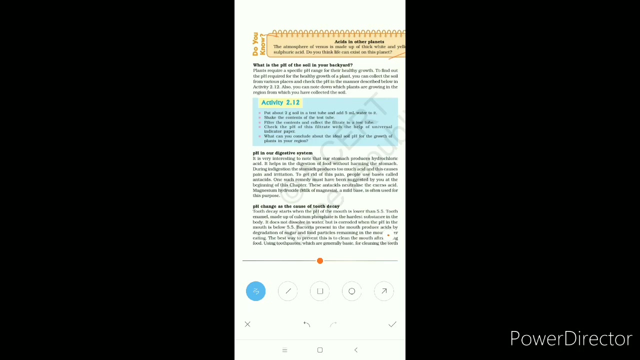 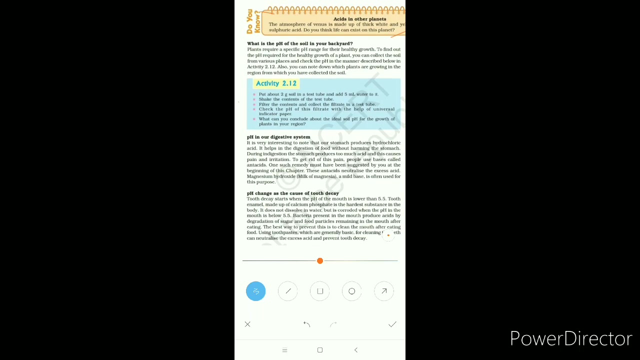 so next what is the ph of soil in our backyard so plants also record a specific ph range for their healthy growth to find out the ph range for the healthy growth of a plant so we have to collect soil from the various places and we can check their ph by taking a little two gram of soil and dissolving in water after that we have to filter this solution and the filtrate have to test with the help of universal indicator paper so that universal indicator paper indicates the ph level by changing the color so if it is acidic then it will show the red color if it is basic then it is so 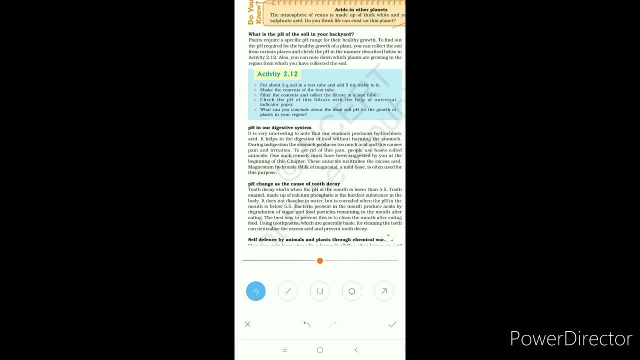 blue in color so next ph in our digestive system 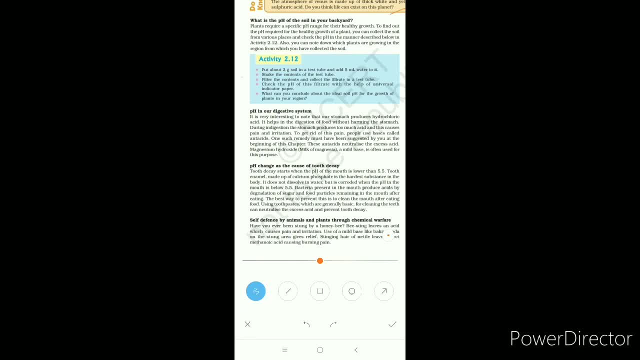 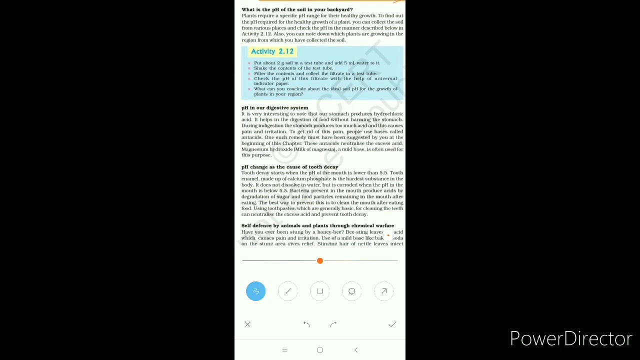 so as we know that our stomach produce hydrochloric acid so this hydrochloric acid helps the food for digestion but sometimes we face indigestion because of excess acid produced in our stomach and this due to this excess acid we cause pain and irritation which is also known as acidity during that these allow us to lose the energy we need so during these times we should take a mild base to get remedy so starting of this chapter we have got one question that when the question is like that when we suffering from acidity problem then what remedy should we take whether we take lemon juice vinegar solution or baking soda solutions So actually the baking soda solution is a base. So baking soda solution is preferable. So it is written here. When we are suffering from acidity then we have to take antacid. So this antacid actually neutralizes the excess acid present in the stomach. Okay. So the antacid may be different types. One is magnesium hydroxide or meal of magnesia. It is a mild base. So when we take this it will neutralize the excess acid present in the stomach. Next pH change as the cause of tooth decay. So tooth decay starts when the pH of the mouth lower than 5.5. Because our tooth is made up of enamel. That enamel is nothing but calcium phosphate. It is a salt and very hard substance. It does not dissolve in water but it will get corroded when the pH of the mouth is less than 5.5. That means when our mouth water is less than 5.5 it will get corroded. After become acidic then the tooth enamel will corrode it and thereby tooth decay will occur. 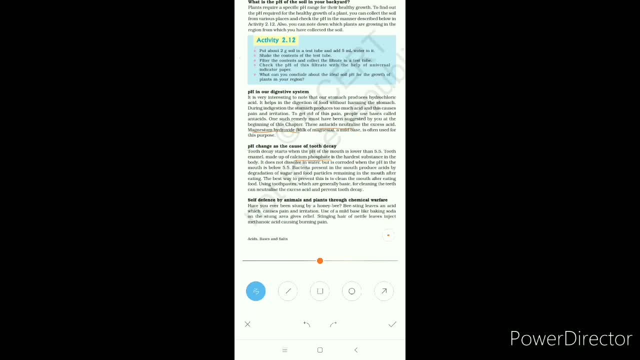 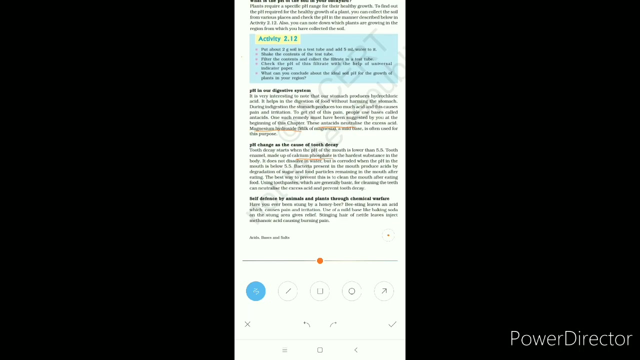 So the acid produced in our mouth is also because of the bacteria present in our mouth that produce acid by the degradation of the sugar and the food particles remaining in the mouth after eating. So the best way to prevent this is to clean our mouth after eating food using tooth paste. Actually tooth paste is generally basic in character. Thereby it will neutralize our acid present in our mouth and prevent tooth decay. 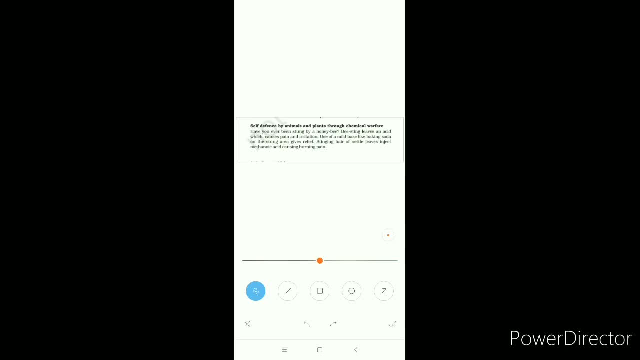 So next cell defense by the animals and the plants through chemical warfare. So plants and animals also protect their own selves, do cell defense through the chemicals. 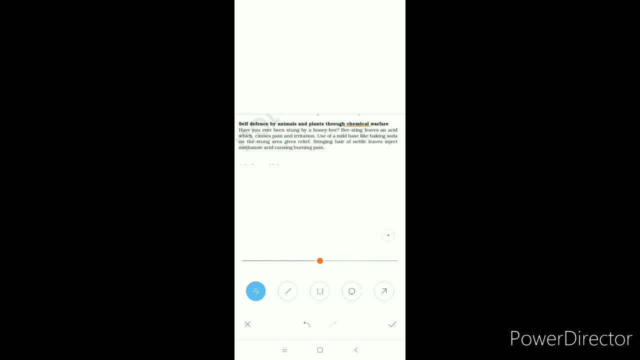 So the chemicals are acidic in nature. If we talk about the honey bee and the red ant, they will release some water softens chemicals through their sting and they cause pain and irritation. Actually that chemicals are acid in nature. 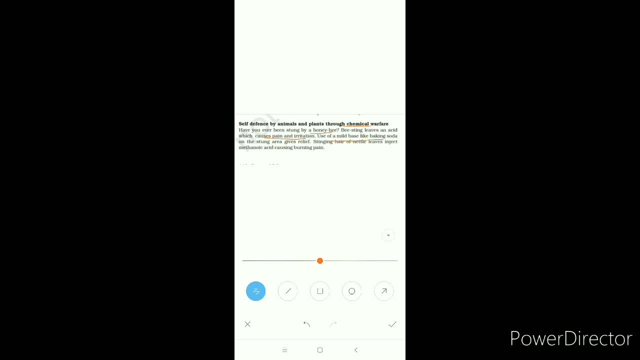 So when we apply mild based like baking soda or oil or 주는 on a piece of cloth. So when we apply mild based like baking soda or oil or sealing on a piece of cloth.